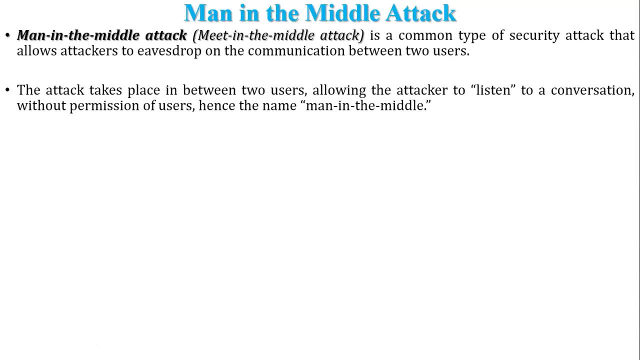 but it will generate a between hacker and attacker. so if the attacker started the attack during the But both the user cannot allow that attacker. But attacker can join this conversation without knowing of user or without permission of users. Hence the name is called man in the middle. 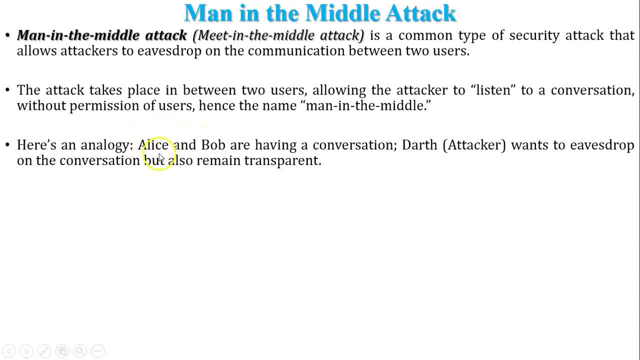 Now here is one analogy: There are two users, One is Alice and second one is Bob. Both are communication with each other. So here we can say Alice and Bob are having a conversation with each other Here Darth- or we can say attacker or hacker- wants to eavesdrop or try to capture the messages on the conversation, but also remain transparent. 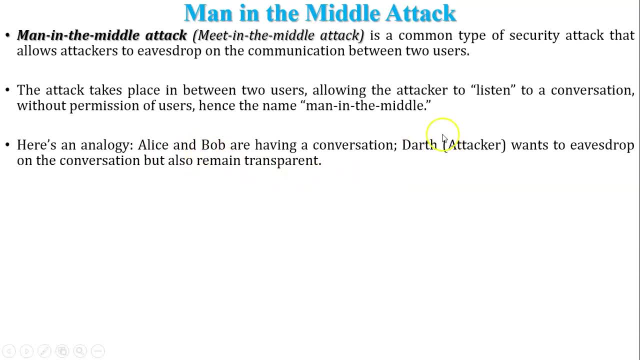 So Alice and Bob both don't have an idea about attacker, can attack or try to listen messages of that conversation. So Darth could tell Alice that he was Bob and tell Bob that she was Alice. We can say Darth, give the identity as a Bob to the Alice. 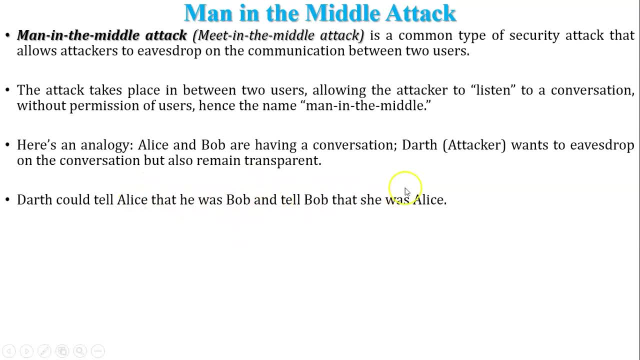 And during communication with Bob it gives the identity as Alice. So this would lead Alice to believe she is speaking to Bob and while actually revealing her part of the conversation to the Darth. So we can say whenever Alice try to send a message to the Bob. 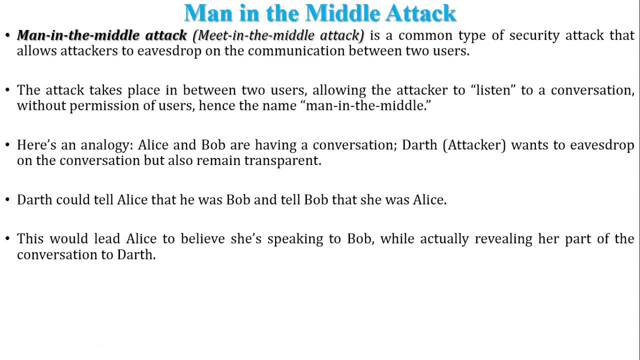 So Darth capture the message, read the message and modify the message. So Alice think that she is already send message to the Bob And same this message. This message is modified by the Darth and send to the Bob Whenever Bob reply to the Alice message. so it is captured by the Darth and modify by the Darth and send to the Alice. 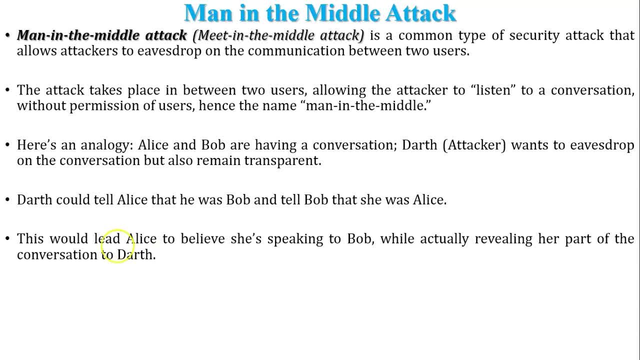 So Alice and Bob don't have an idea about that. there is one attack in between the communication, So Darth could then gather the information from this conversation and alter the responses and pass the messages along to Bob, Who think he is talking to Alice. So we are already discuss about that. 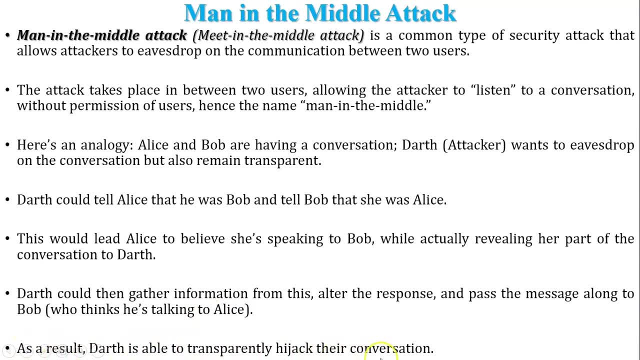 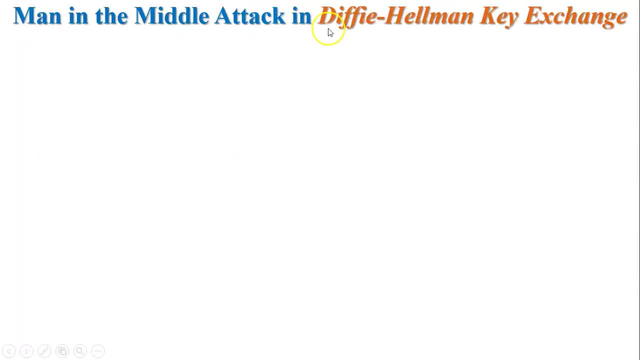 As a result, Darth is able to transparently hijack their conversation. So this is one scenario of the man in the middle attack, Now man in the middle attack in Diffie-Hellman key exchange. So before discuss about this attack in Diffie-Hellman key exchange, 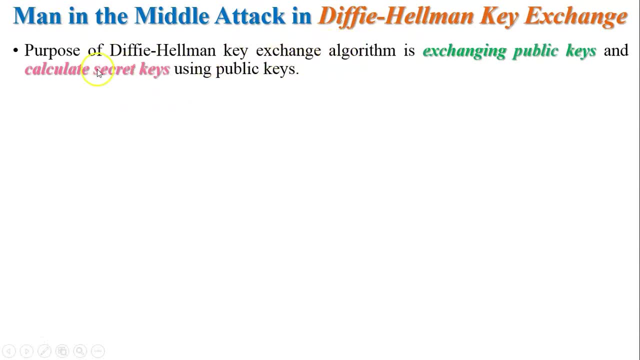 So before the what is the purpose of Diffie-Hellman key exchange? I will revise this purpose. In Diffie-Hellman key exchange algorithm is used to exchanging public keys and calculate secret keys Using that public keys. Then subsequent messages or subsequent conversation, or we can say further communication, are encrypted using the secret keys. 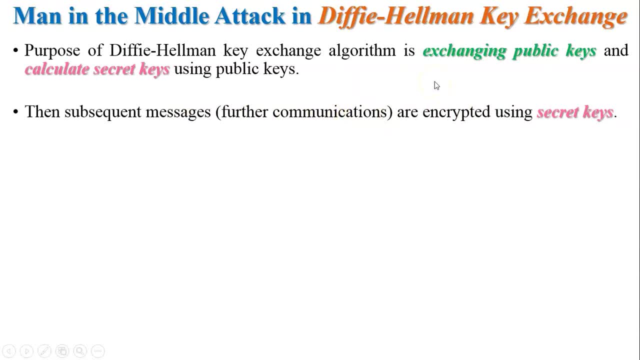 So mostly used to exchanges key and generate secret keys. So how? man in the middle attack take place in the Diffie-Hellman key exchange. Man in the middle attack in Diffie-Hellman key exchange is take place during the exchanges of public keys. 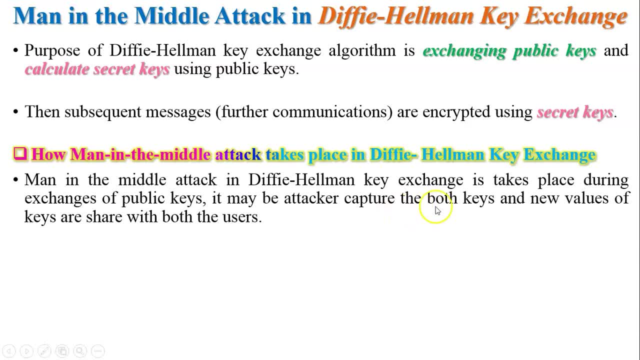 It may be attacker capture. the both keys and new values of keys are shared with both the users. So we can say whenever Alice or Bob, or we can say any of the user- want to communicate with each other And they want to use secret key. 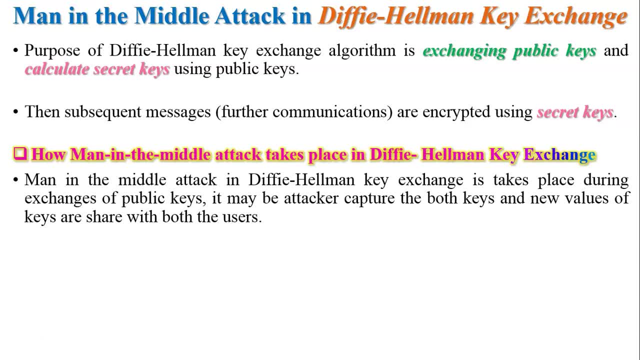 So before calculate a secret key, they are exchanging public keys as per the Diffie-Hellman key exchange. So during exchanges of that public keys In mate in the middle or man in the middle, attack Attacker can capture this public keys And new public keys given to the both the users. 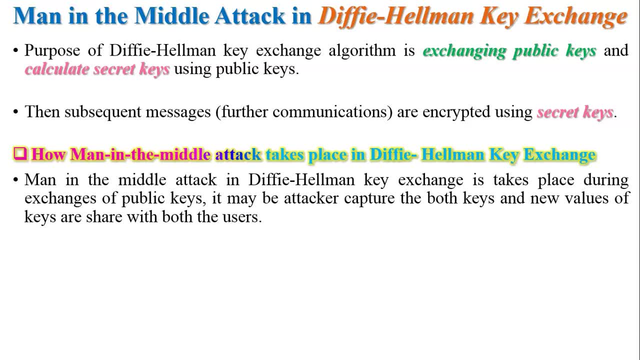 But both users don't have an idea about that. So subsequent encrypted messages are read and modified by the attacker, Because attacker calculate the secret key with the help of that public keys Then send to the respective users. Using this, attacker may read and modify messages and get the benefits of the user communication. 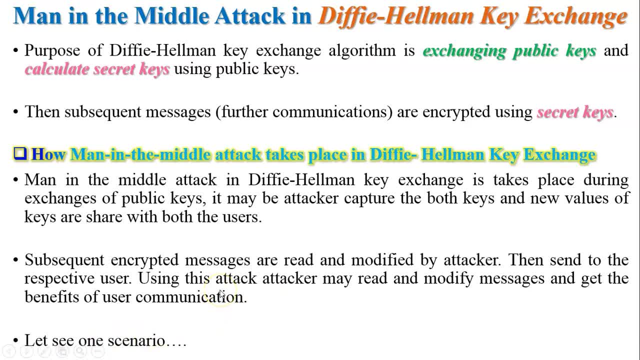 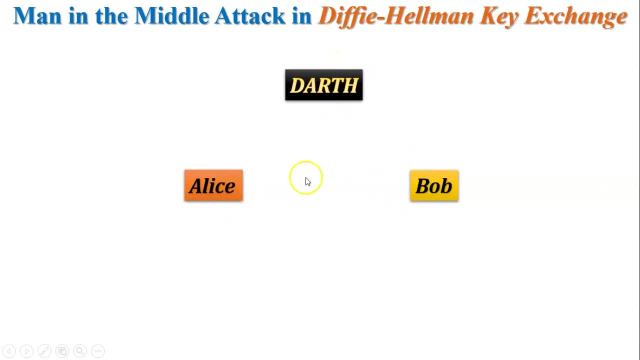 So let's see one scenario, how it take place. So in this figure you can see this is Alice, this is Bob and this is Darth. So Alice and Bob wants to communicate with each other. So before communication, they want to calculate their secret key. 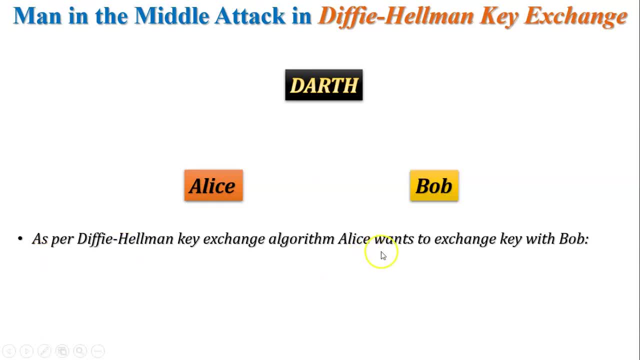 So, as per the Diffie-Hellman key exchange algorithm, Alice wants to exchange the key with Bob. So, before exchanging the keys, Alice select XA. This is private value. Now calculate YA based on XA. Now you can see this equation. alpha raise to XA, mod Q. 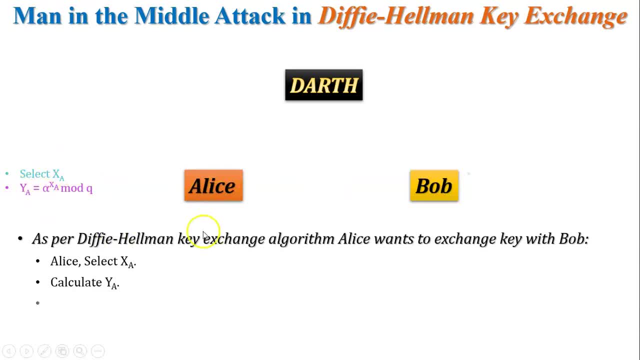 Now, YA is the public key and it is shared with Bob. Now, same Bob, select XB. XB is the private value And calculate YB from the value of XB. Now see this equation: YB is equal to alpha. raise to XB mod Q. 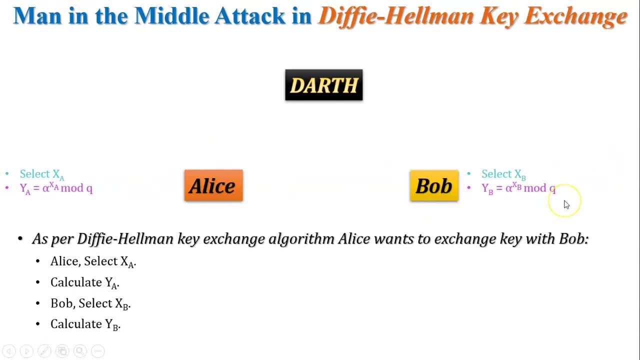 So, based on this Diffie-Hellman key exchange algorithm, both are calculate public keys, or we can say public values, YA and YB. Now both are transfer, both the public keys. Now Darth prepares for the attack, So Darth can generate two random private keys, XD1 and XD2.. 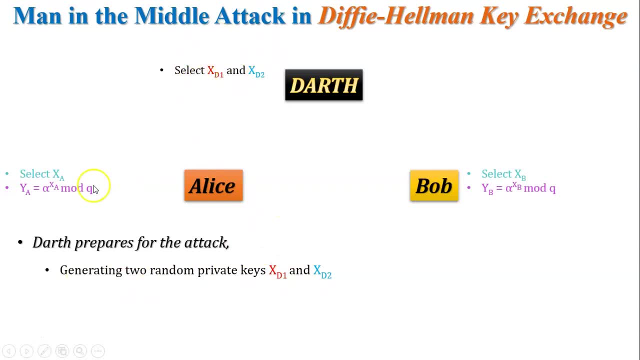 Now you can see over here: this is XD1 and XD2.. So same as the XA and XB. So calculate public key YD1.. So it is based on XD1.. Now calculate the public key YD2.. It is calculate from the XD2.. 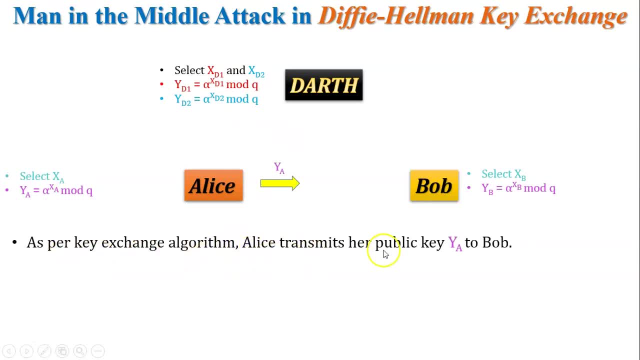 Now, as per the key exchange algorithm, Alice transmit her public key YA to Bob. Now see in the figure: Alice share his public key YA to the Bob Before Bob capture or Bob receive this key. So Darth intercept YA and destroy the message And YA, or we can say public key of Alice is captured by the Darth. 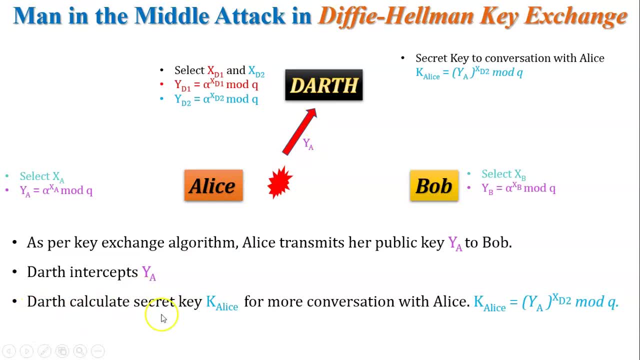 So, based on this, YA Darth calculate secret key K Alice for more conversation with the Alice. So this is K Alice is the secret key which is used to conversation with Alice. So K Alice is equal to YA raise to XD2 mod Q. Now you can see over here this is the equation for the secret key, or communicate with Alice. 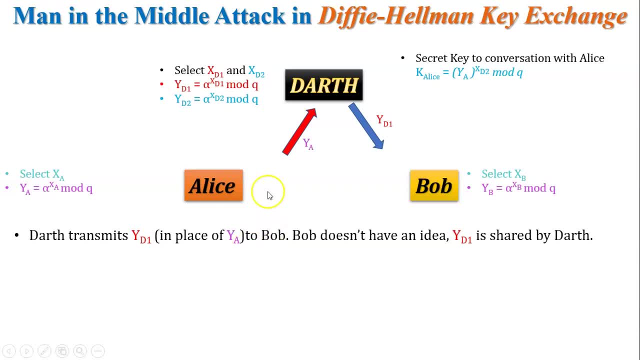 Now Darth transmit YD1 in place of YA. YA is captured by the Darth and new value: YD1 shared with Bob, So Bob doesn't have an idea. YD1 is shared by Darth, So Bob receive this message and consider: is YA. 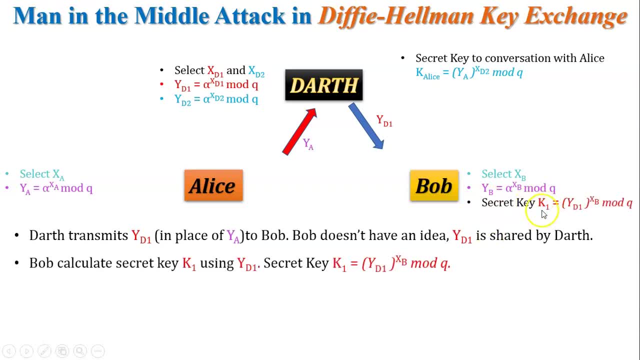 So now what happen? So Bob calculate its secret key. Now here you can see this is: K1 is equal to YD1. raise to XB mod Q. So this secret key, K1, will be calculate from the value of YD1.. Now Bob transmit his public key, YB, to Alice. 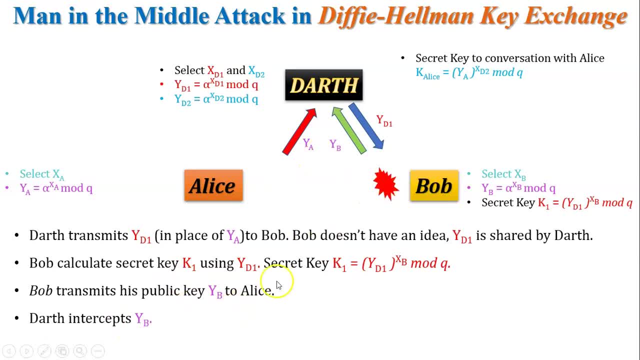 So Darth intercept YB and destroy the message. So again Darth calculate secret key K Bob. Here K Bob, you can see over here for more conversation with Bob. So this is the secret key of K Bob is equal to YB. raise to XD1 mod Q. 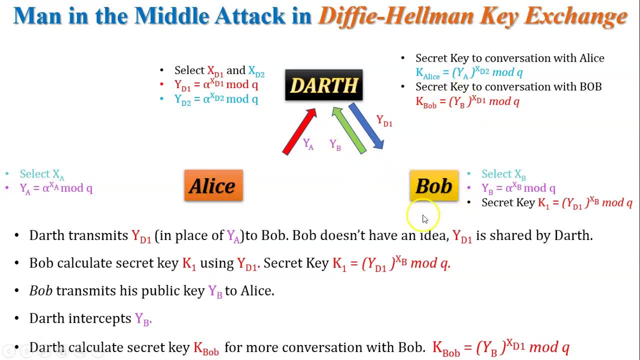 So it is calculate from the value of YB and YB value given by the Bob. Now you can say K, Bob and K1. both are the same value. So here secret key is the same: K, Bob and K1.. So Darth and Bob communicate with each other using this secret key: K, Bob and K1.. 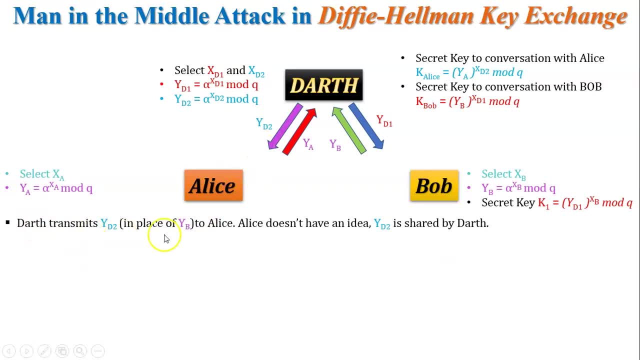 Now Darth transmit YD2 in place of YB, because YB is captured by the Darth. So, in place of YB, YD2 is shared with Alice, But Alice doesn't have an idea. YD2 is shared by Darth, So what happen? 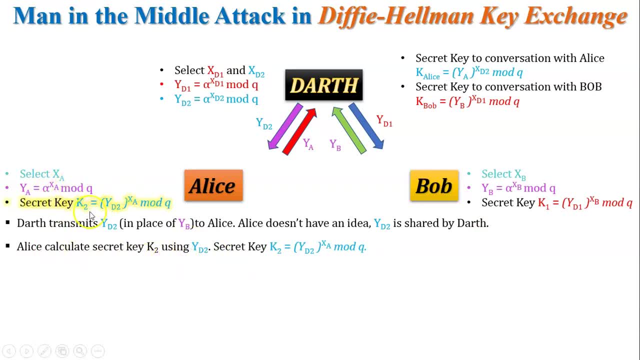 Alice. calculate the secret key K2 using YD2.. Now you can see this is: K2 is equal to YD. raise to XA mod Q. So value of K2 is same as the K Alice. So using K Alice and K2, both are the same secret key. 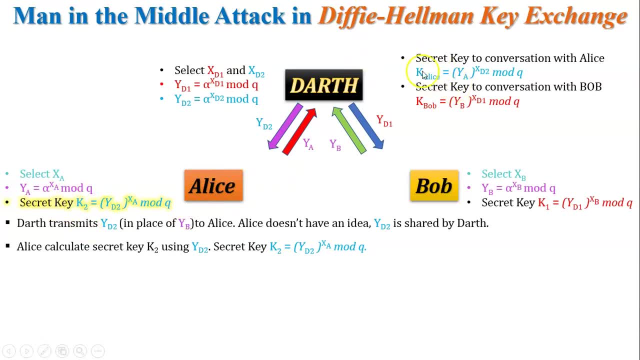 So Alice and Darth communicate with the K2 and K. Alice And Darth and Bob communicate with K Bob and YB. Now Darth will capture all subsequent messages of Alice and Bob, Read and modify all the messages and send to the Alice and Bob. 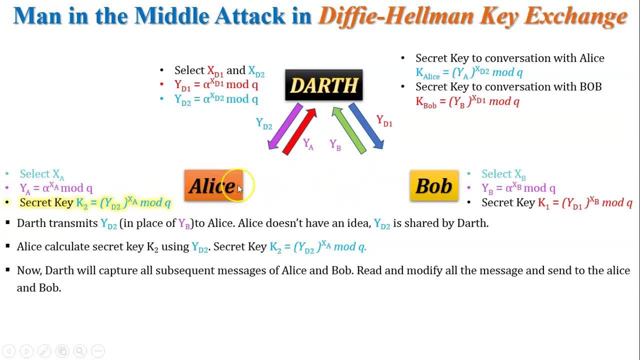 So what happen? So whenever Alice want to send the message to the Bob, So at that time Alice message is encrypted using K2. So captured by the Darth. So Darth decrypt that message using K Alice, Modify the message and encrypt by K Bob and send to the Bob. 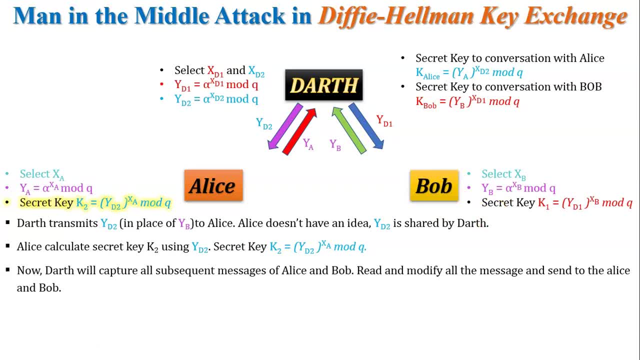 And again, Bob will receive that message. But Bob have no idea. this message is modified and send by the Darth. So what happen? Bob will receive that message and decrypt using K1.. And it gives the reply. and same thing happen during the reply by the Bob. 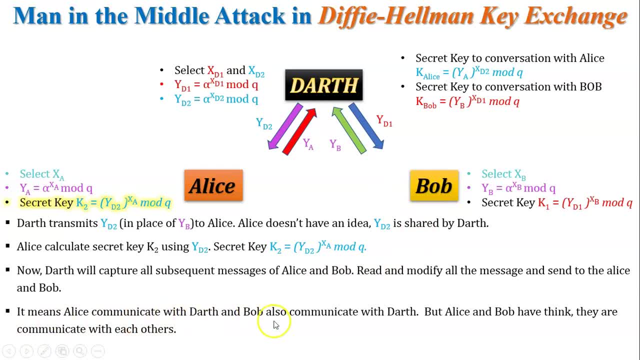 So it means Alice communicate with Darth and Bob also communicate with Darth. But Alice and Bob have thing: they are communicate with each other. It means Alice and Bob have no idea this messages are captured by the Darth. So this type of attack is called man in the middle attack in Diffie Hellman key exchange.